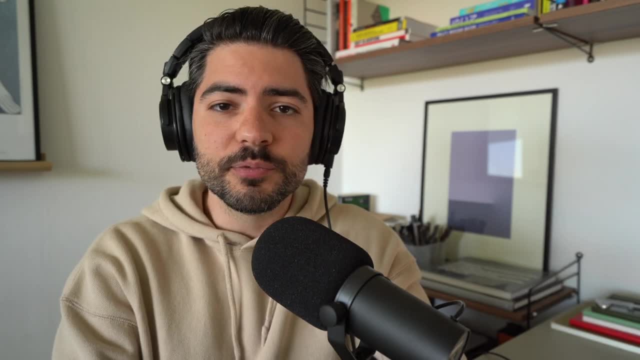 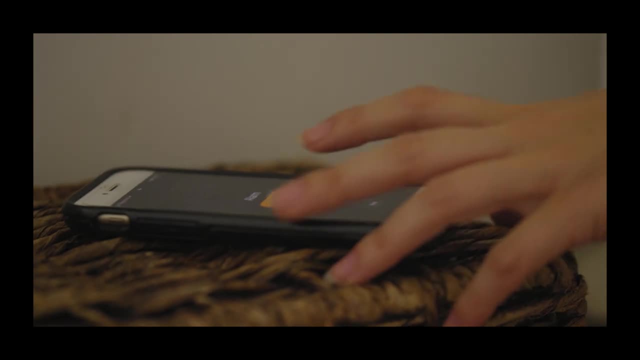 to this episode. you are also performing some kind of human computer interaction. Even in our sleep we interact with computers. you know, some of us measure our sleep with smart watches or rings and most of us actually wake up to some kind of digital alarm clock. This phenomenon of HCI, the 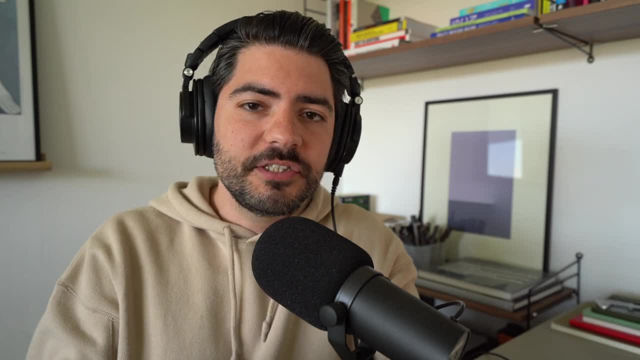 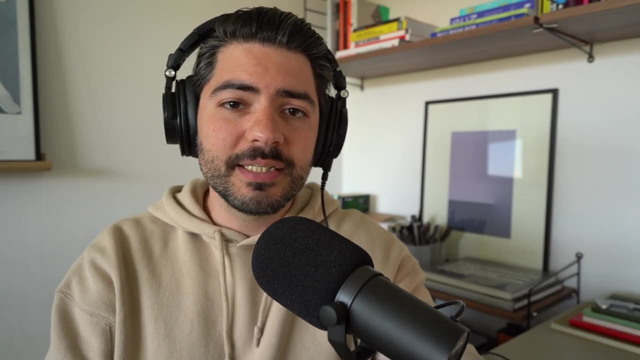 experience of it is everywhere. it is the defining feature of human life today. This is HCI as a phenomenon, it's the fact that we live with computers, and it's not only these keyboard and mouse and screen kind of things, but anything that involves digital components: your dishwasher, your. 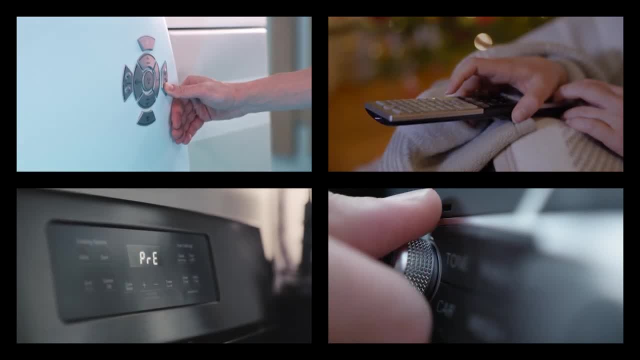 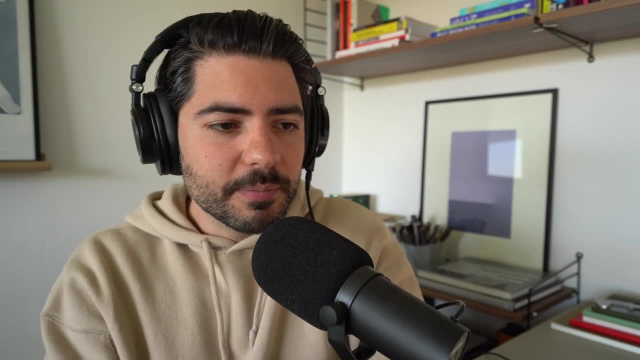 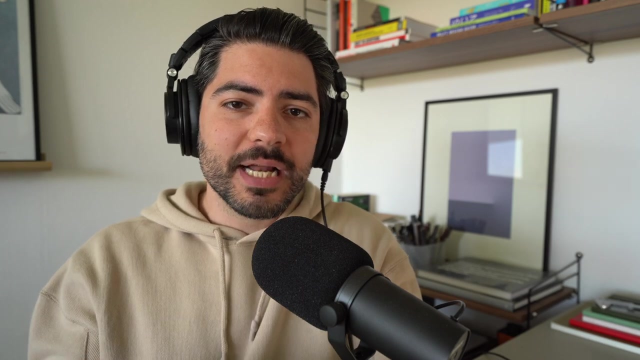 tv, your car. But when you hear people talking about HCI, it's probable that they are not only talking about the phenomenon of using a computer, but rather they are talking about a profession or discipline Which deals with this phenomenon. So human computer interaction is the name of what happens. 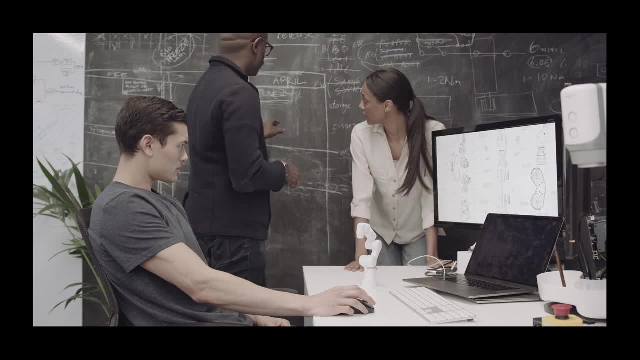 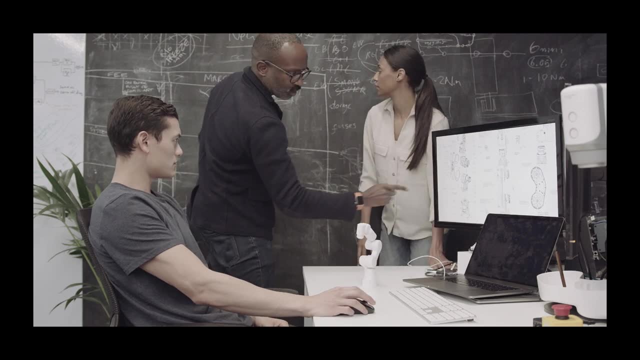 but it is also the name of the scientific and professional field where people have the job of analyzing it and designing it. This, the scientific and professional discipline that is called HCI, is what we're going to talk about in this episode of design discipline. My name is Mehmet Aydin Baytash. 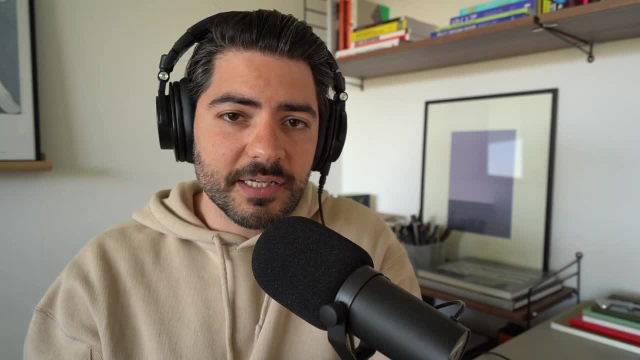 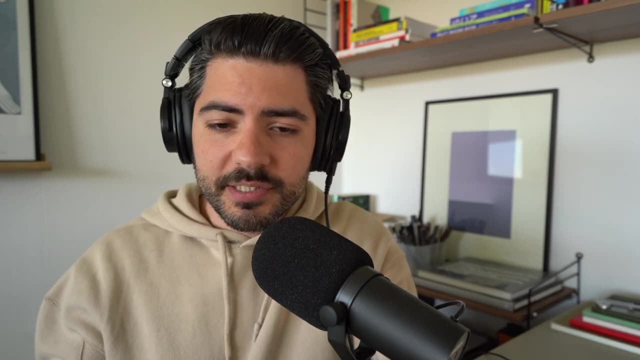 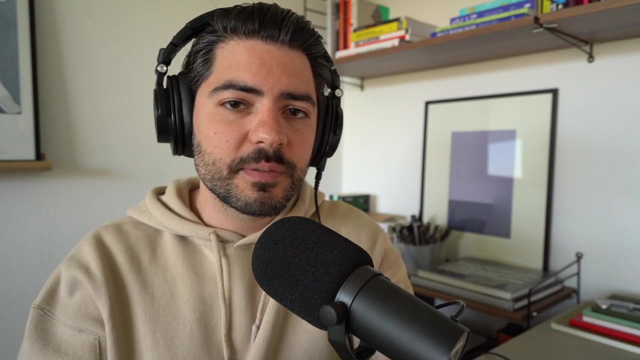 I'm a scholar of design and technology and research in HCI is basically my job. I design and develop HCI applications, I write about HCI, I manage research projects. I teach HCI at the university and I feel incredibly privileged to be working in this field, because computers and the ways that we use them are 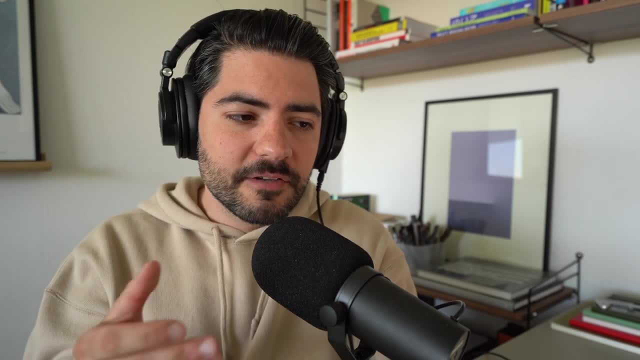 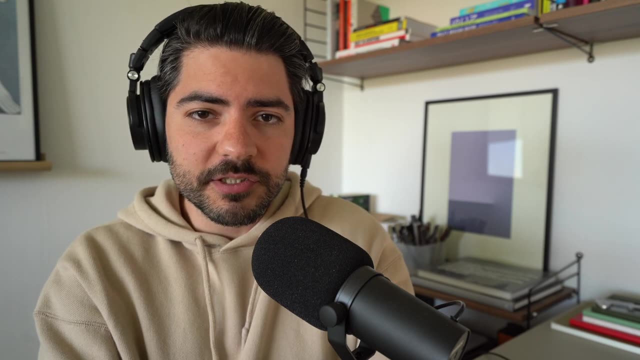 essential to our lives. HCI is basically the defining feature of human life and culture today and naturally there's a lot of interest in HCI as a profession. A lot of people are interested in getting HCI related jobs. Companies are looking for hundreds of different kinds of professionals. 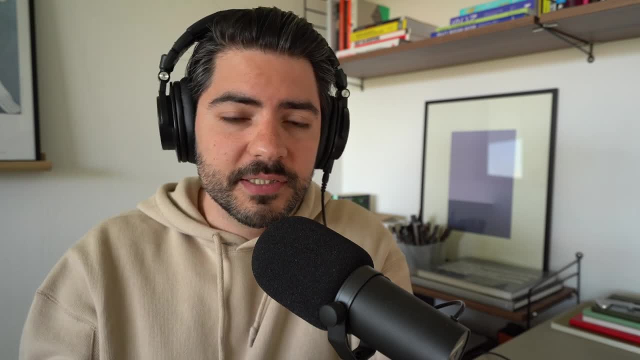 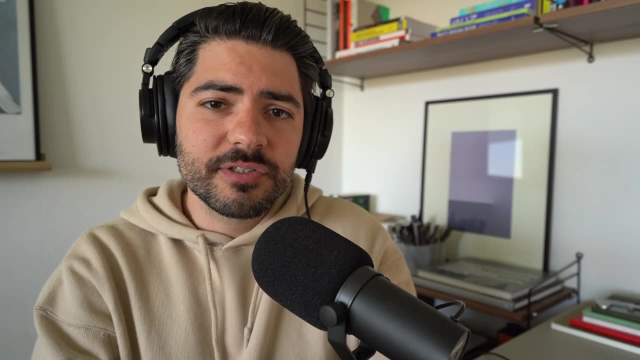 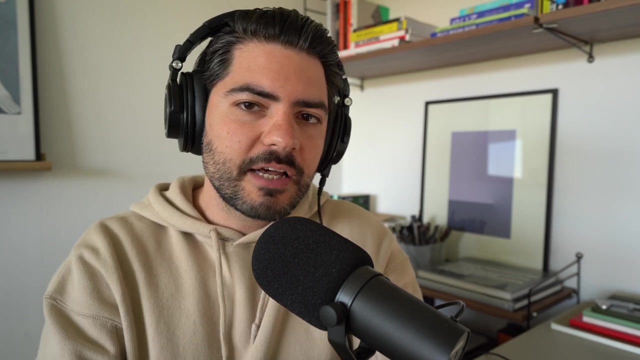 that have to do with computing and design and user interfaces. In the world of academic research, where getting funding is a significant challenge for all of us, HCI researchers are actually treated a little more generously compared to our colleagues in like social sciences or the arts. However, compared to the level of 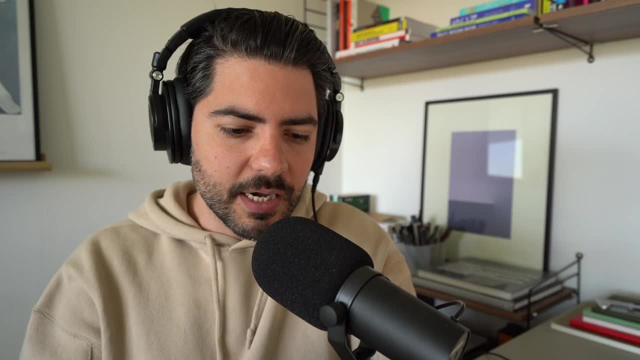 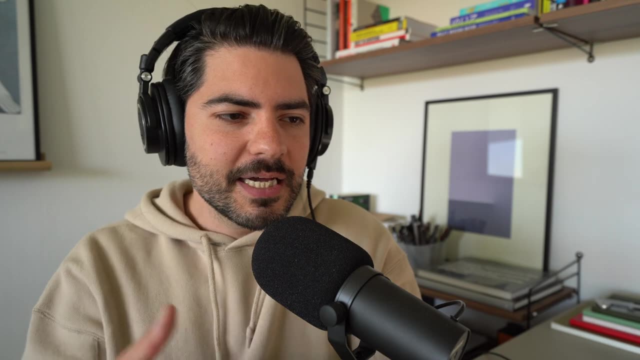 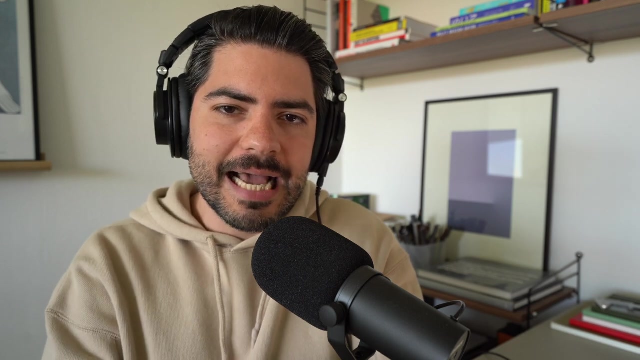 interest and the relevance of the phenomenon of HCI. the actual profession of HCI is quite small and it's quite challenging to get into and the challenge here is largely because a lot of people, when they start out, don't have a mental model of HCI as a scientific field which has enough detail and enough clarity. 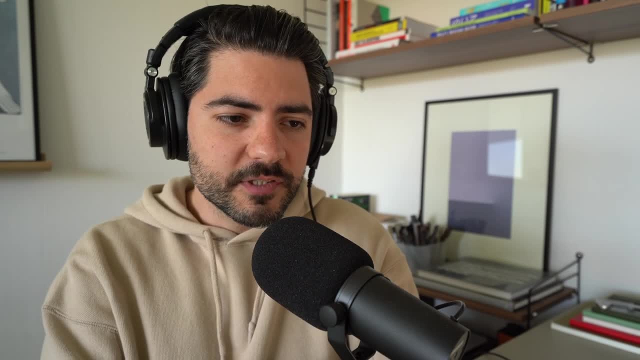 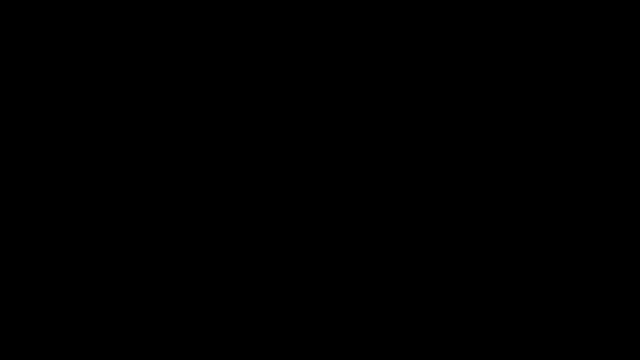 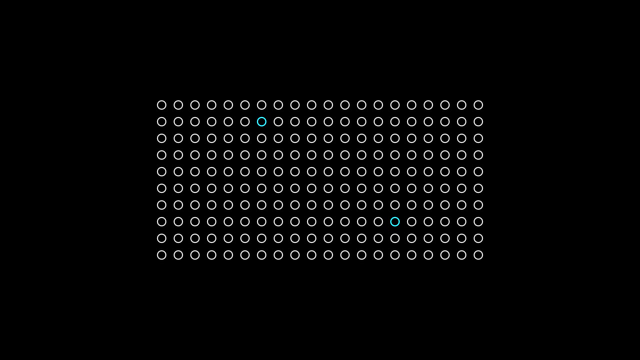 I'll give you an example. Around a year ago, I was involved in a university project and I teamed up with two professors and we had the job of hiring two HCI researchers. We had two positions for PhD researchers and we got more than 200 applications for these positions. Most of the people who applied 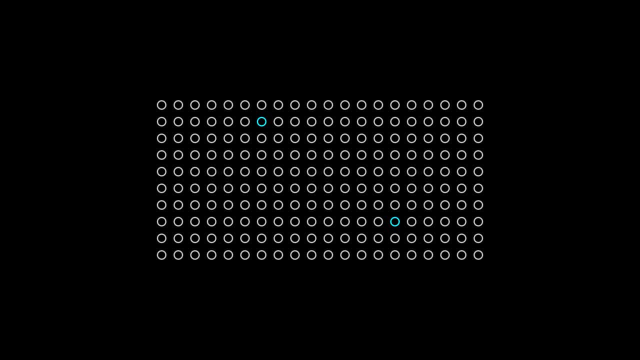 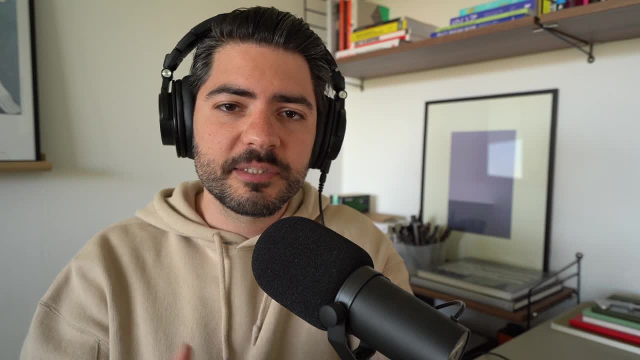 were very smart and very successful. Some of them were great engineers, Some were designers, entrepreneurs and different kinds of scientists. Very smart people, Very cool skills and experiences that they brought. But out of 200 people, most of whom were very impressive. 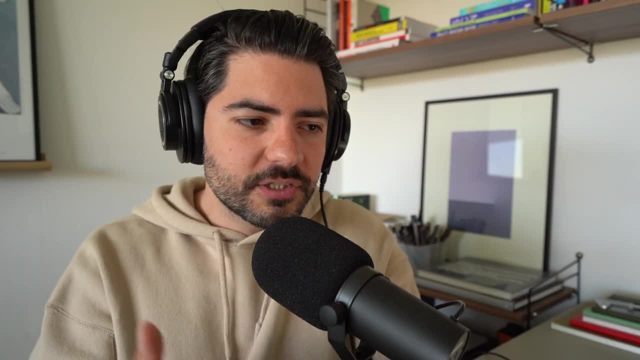 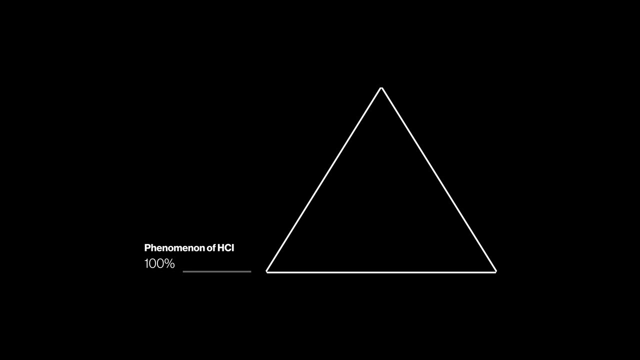 there was only like 10 of them who really understood the field of HCI. So they all understood HCI as a phenomenon and most of them understood the essential ideas, the ideals of HCI as a scientific and professional field, but only around five percent of them actually. 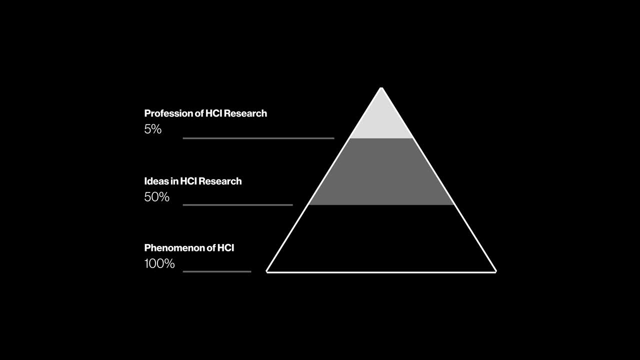 actually understood the boundaries and the landscape of HCI in terms of its existential facts And, naturally, those people were the ones that we interviewed for the jobs. So what I'm going to talk about now is going to help those of you who are interested in HCI. 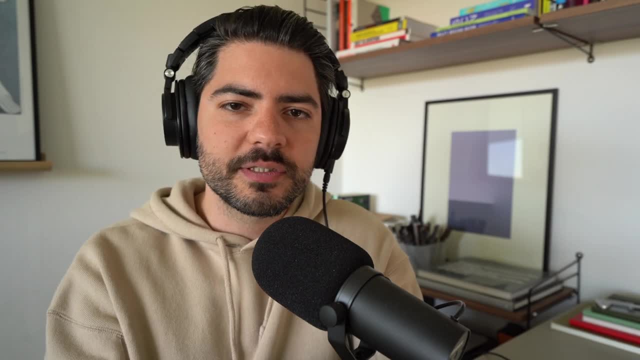 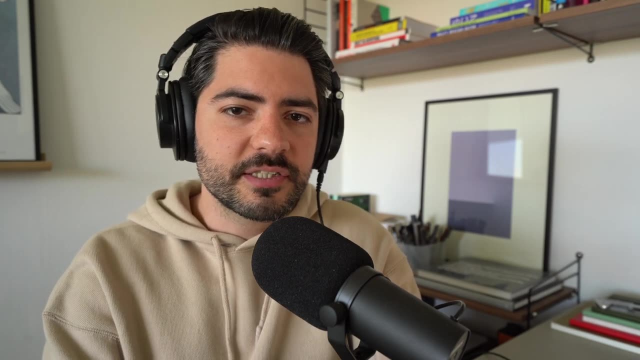 as a profession, especially those of you who are looking at graduate studies and especially PhD programs in HCI, And there are two reasons why we focus on this. The first is that a few days ago, I actually posted on Twitter asking the community for what questions to cover in this. 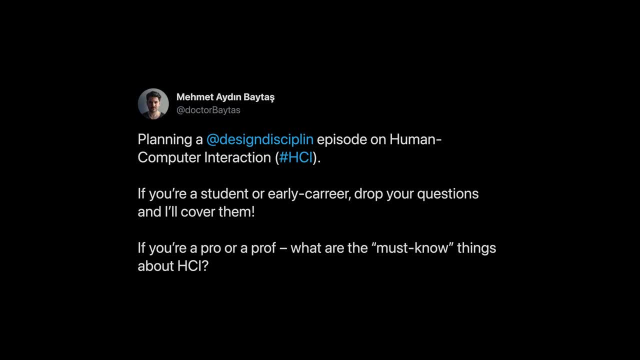 episode about HCI And one of the most salient requests was to talk about how to get into HCI PhD programs. So, with a shout out to Faria and others who submitted questions, we're going to talk about some of the concepts you need for this exact purpose. The second reason why this is 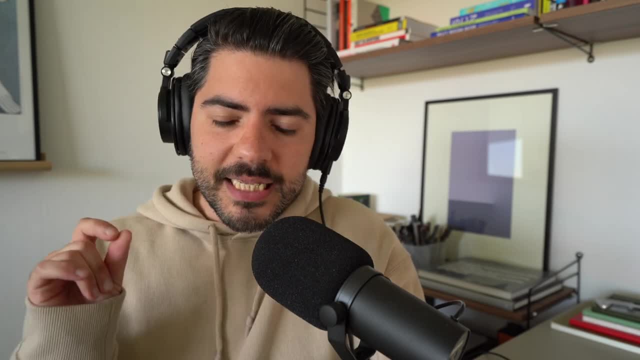 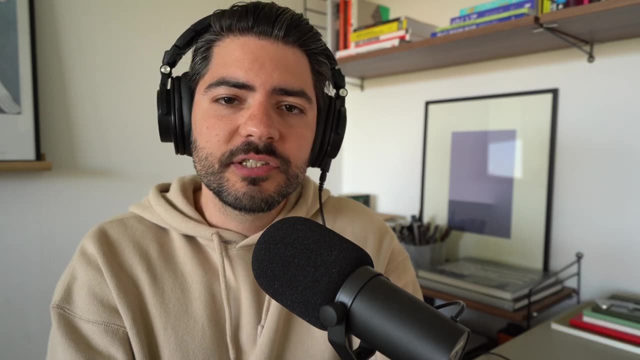 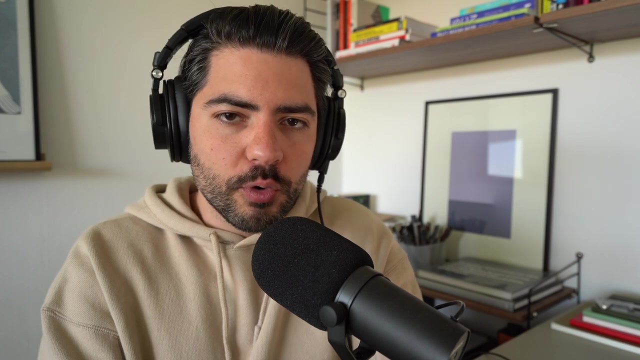 especially relevant to PhD studies is that, in fact, even though the phenomena of computers are everywhere in our lives, HCI as a profession actually refers to a very particular niche within academic and scientific research, And this is my first point. There isn't really a job or position that is. 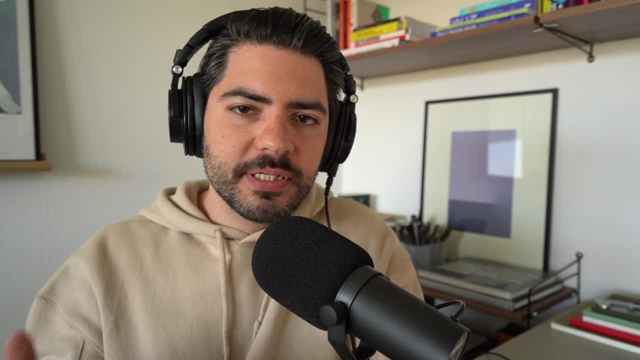 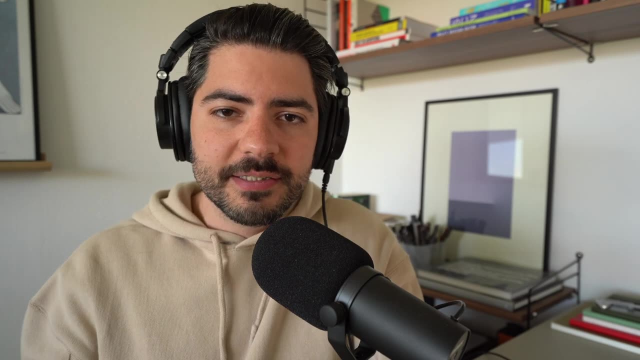 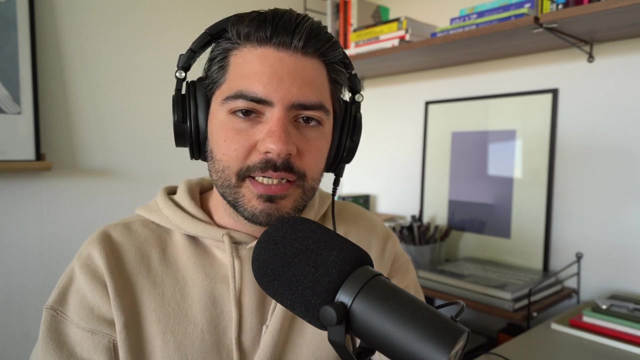 called HCI, which exists purely in the world of business, at companies. In this way, it's different from other jobs like being a programmer or engineer or graphic designer or psychologist, because even though many universities have these programs where you can study HCI, jobs like HCI designer or HCI manager or things like that don't really. 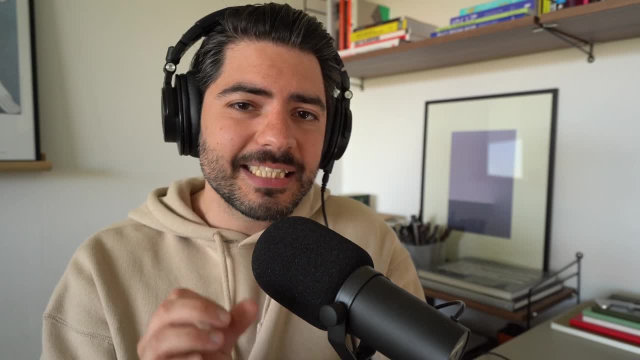 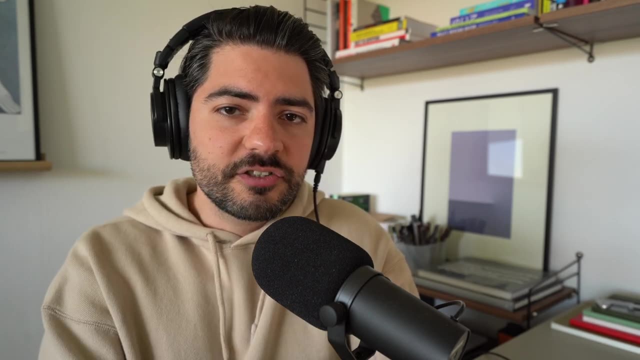 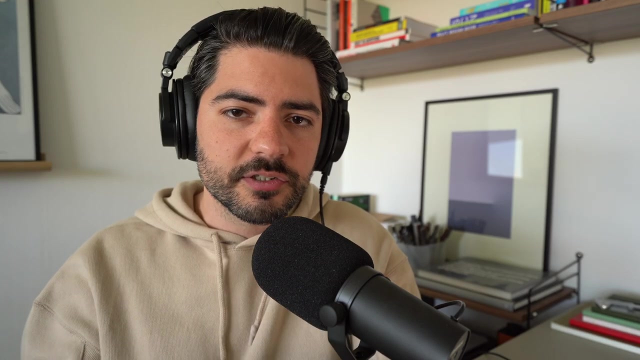 exist. Basically, the only job where you would have HCI in your actual job title in an actual company is the job of a HCI researcher, And these jobs are really rare. They basically exist only at these large tech companies with big budgets for innovation and research. In fact, I went on. 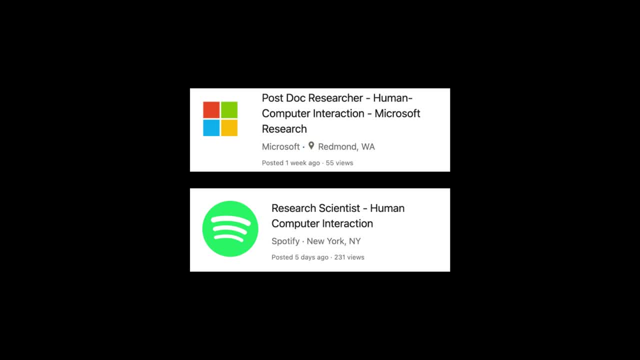 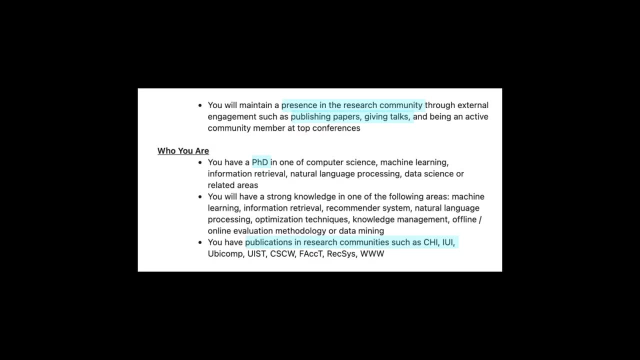 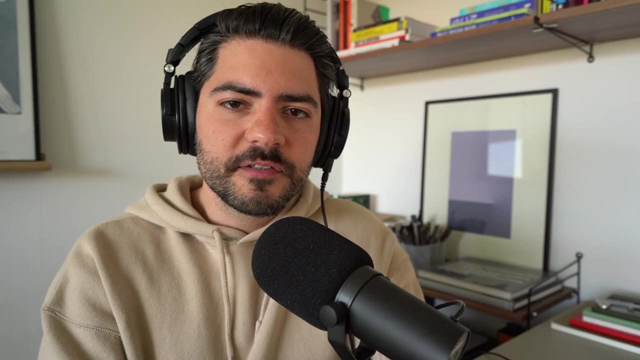 LinkedIn to search for these jobs and found only two of them among them. So I'm going to show you some of the jobs that you should have a PhD and you should have published your research at particular scientific conferences and journals. And this is the first thing that confuses people. 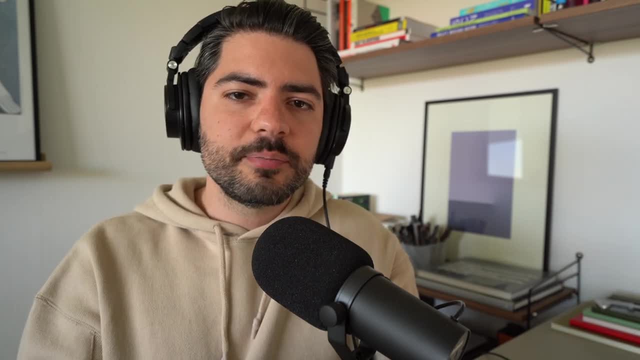 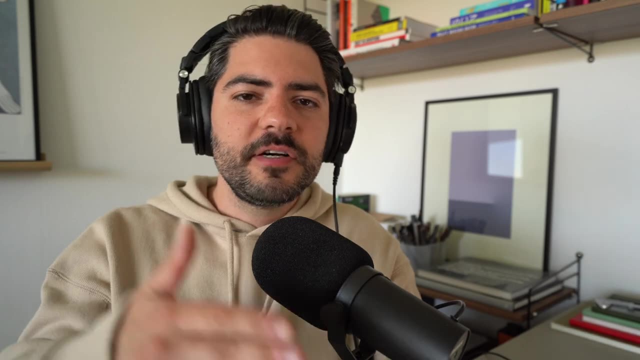 because the essence or the ideal of HCI is very broad. You know, if you go to any other resource, like various books and lectures and whatnot, usually they will hit you with a very long and very complicated definition. Wikipedia will tell you, for example: 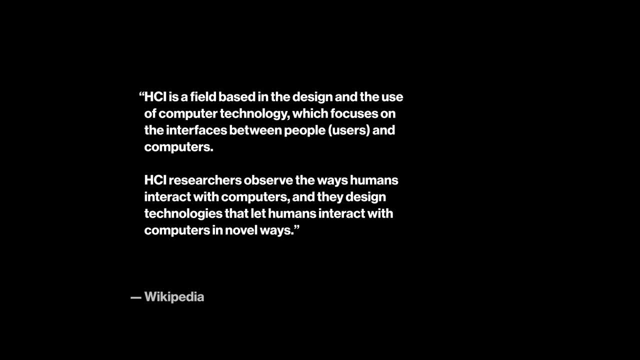 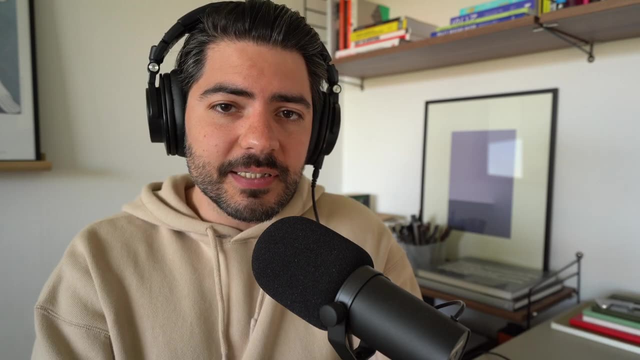 that HCI is a multidisciplinary field of study based on the design and use of computer technology and, in particular, the interfaces between computers and users. It's very broad, It's very inclusive, It's trying to do justice to all that HCI is and all that it could be, But the reality. 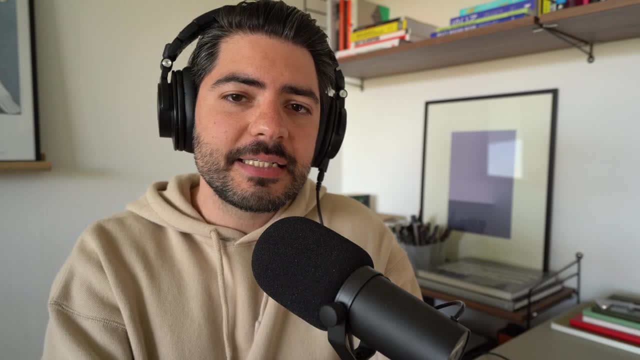 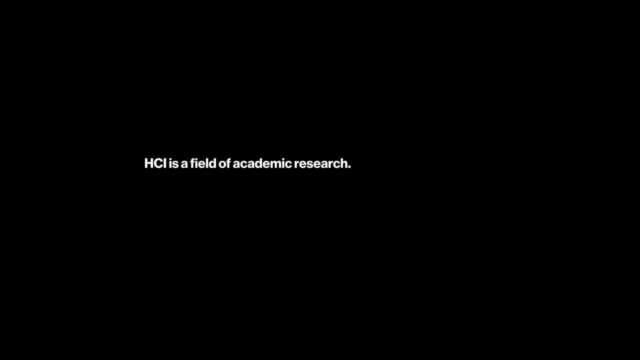 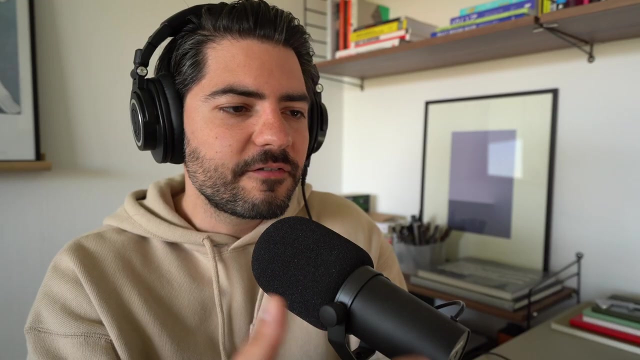 the existential fact is that HCI is the name of a very particular niche in scientific and academic research, So this is the first thing that you need to understand if you're looking for a job: HCI is a research discipline and therefore it is subject to all of the concerns and constraints. 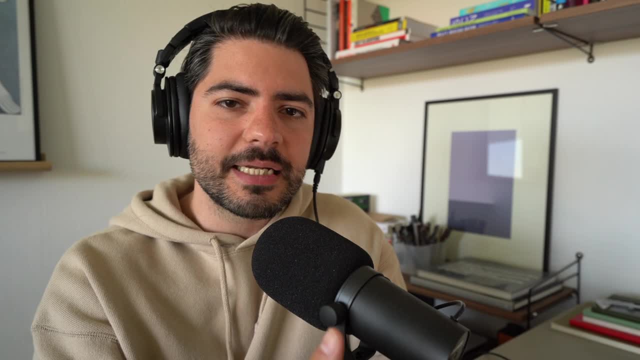 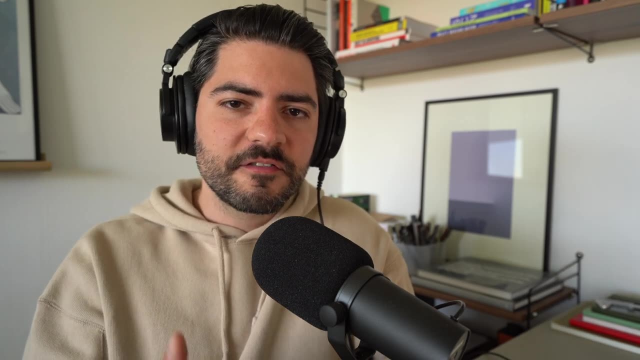 that apply to all kinds of like scientific and academic research disciplines. So if you want to become a HCI researcher, you kind of have to be interested in like the rigor and philosophy of science and academia. You will need to read thousands of research papers and write a lot. 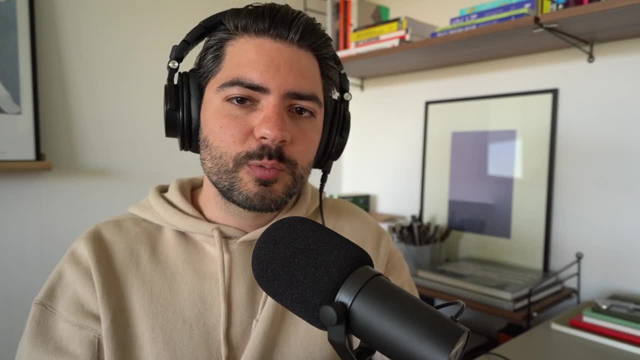 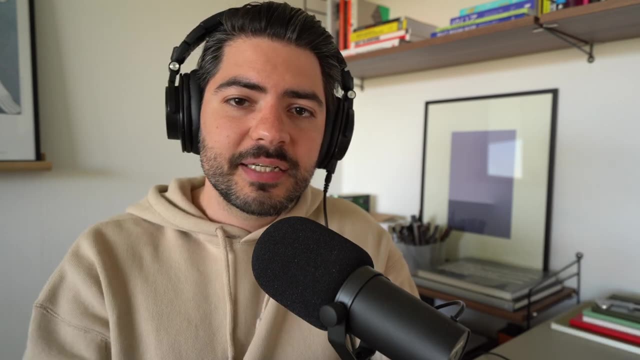 of your own. You need to engage with the academic world, with the ecosystem of like universities and academic careers and research funding and conferences and journals. You might have to teach courses and give lectures And all of this is actually going to take up most. 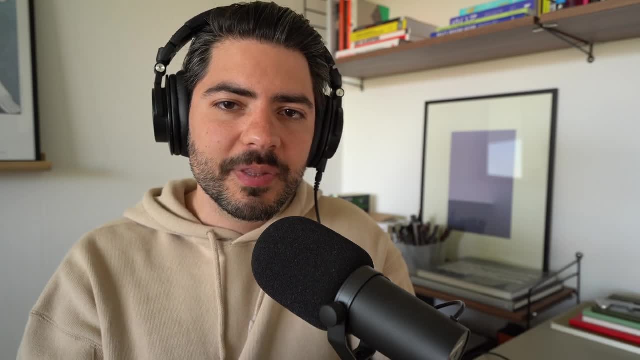 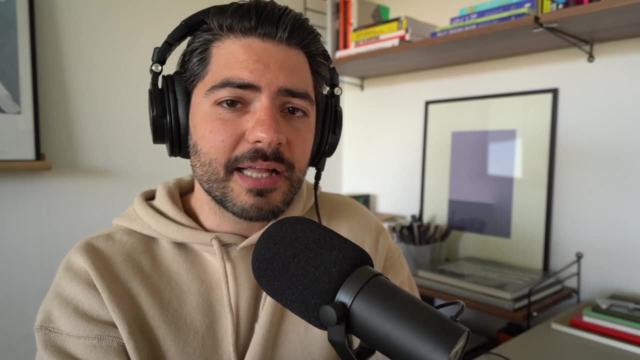 of your time, to the extent that you will have very little time left to create actual products. Most professional HCI researchers actually don't design anything in a hands-on fashion. They don't develop a lot of software. Now, there are exceptions to this, For example, 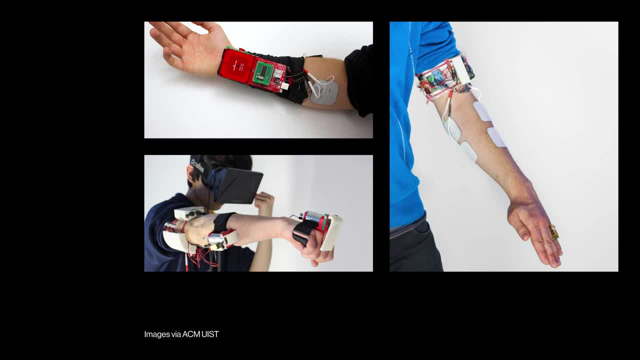 there is a HCI research conference called User Interface, Software and Technology, or UIST, where a lot of technical and tactical work is presented, And there are some design related venues as well, But on the vast majority of these projects, the people who are doing this 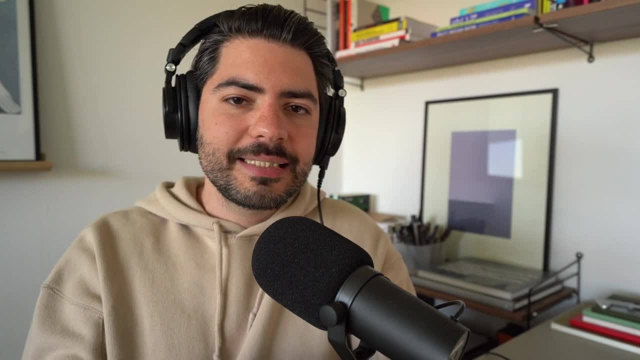 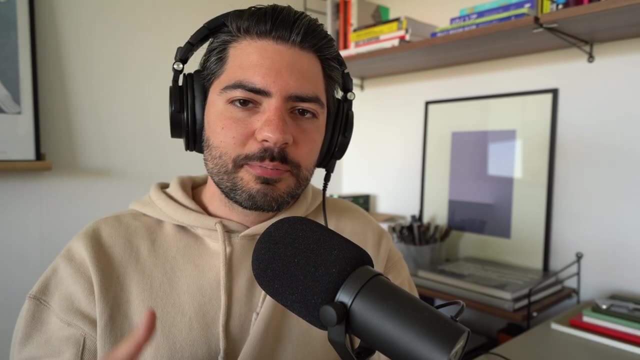 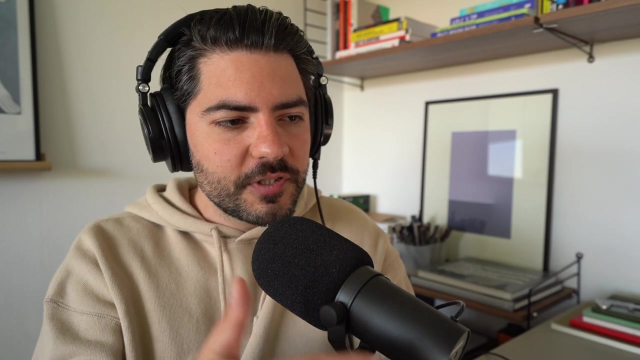 hands-on work are actually graduate students, So it's only at the earliest stages of this career where you will actually get to do the hands-on work. Later, as a professional HCI researcher, you might be on a team where you collaborate with people who do these things. But your job 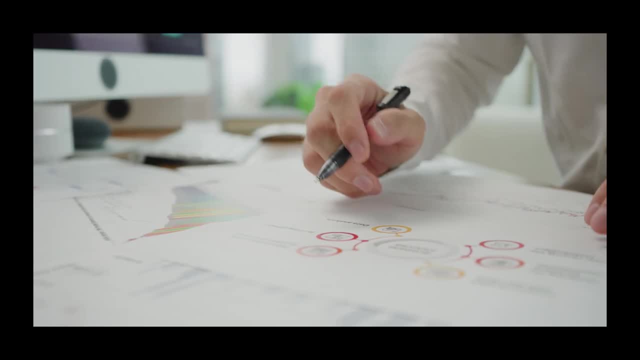 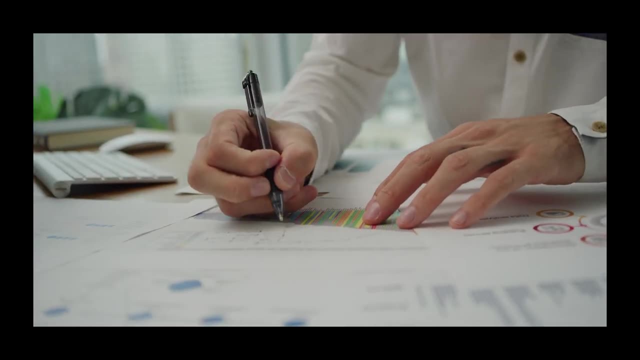 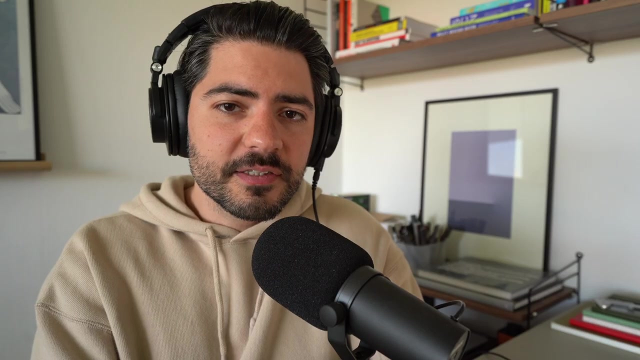 will not be to design user interfaces and to develop different gadgets. In fact, your job as a HCI researcher is much closer to being an analyst, a critic, a teacher, a philosopher and even a project manager, much more than it is to being a designer or developer. This is the first thing. 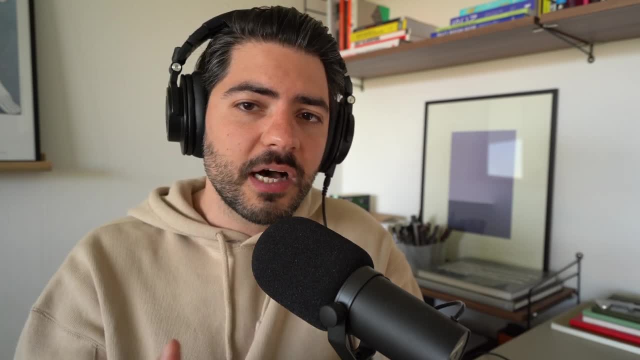 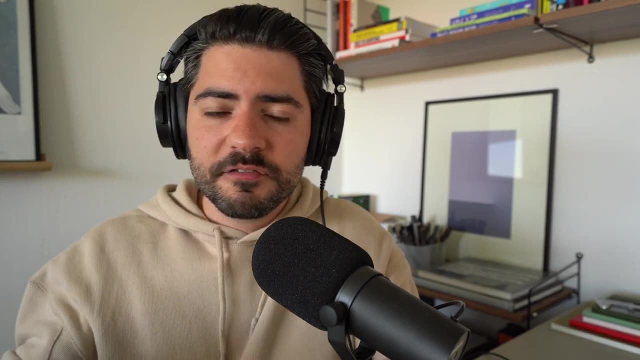 that you need to clear up if you're interested in HCI as a profession. A lot of people who think they are interested in HCI are actually more interested in design or development, which are different disciplines. These jobs do have some overlap, since they basically deal with the same subject matter of 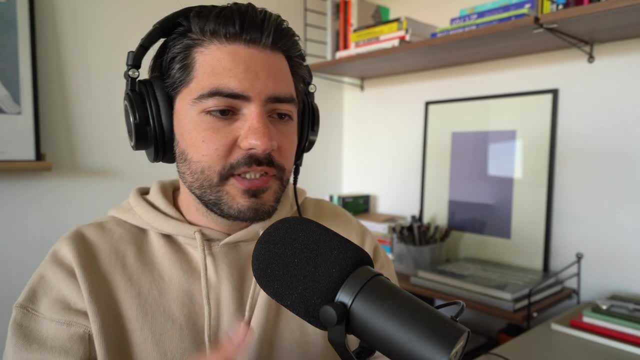 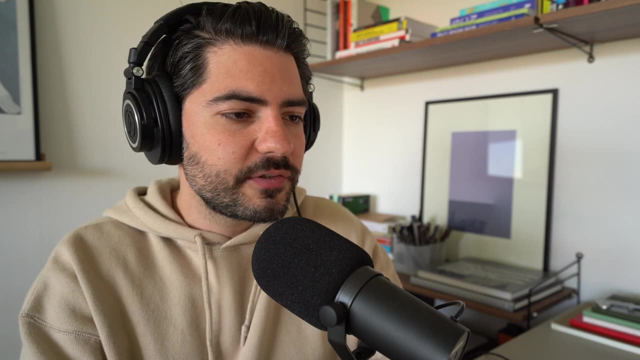 user interfaces. They are definitely related. Researchers, designers and developers very often work together in teams. A lot of people switch between these jobs at various points in their career, And you can definitely get an education in one of these things and get a job in the other. 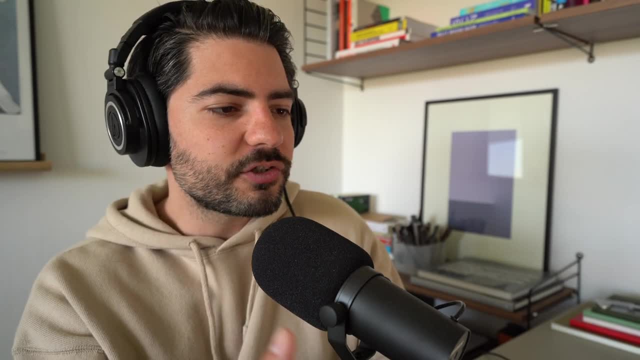 In fact, if you study HCI, it will lead you to a lot of different jobs in product design or engineering or marketing, sales, user experience research. But the work that you would do as a HCI researcher is much more complex than the work that you would do as a developer. 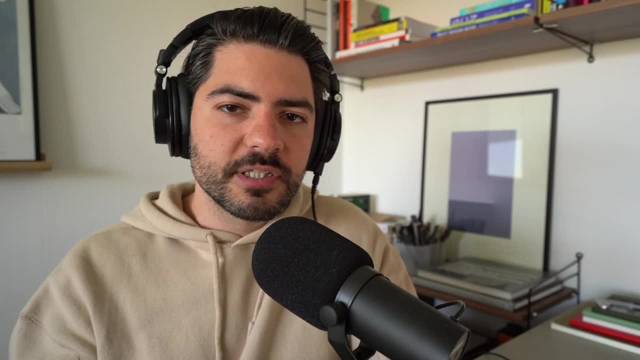 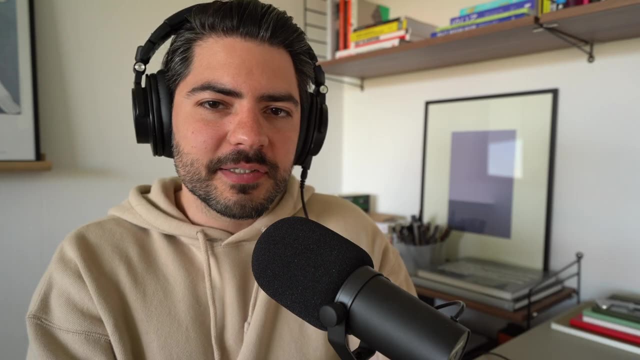 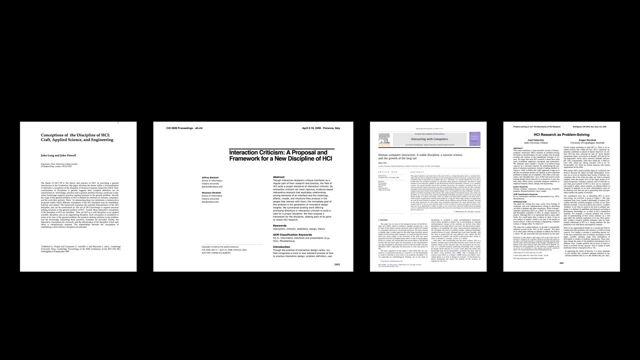 As a professional HCI researcher is different from those, and it's very specific. So what, then, is the actual work that a HCI researcher does? Now, the answer to this gets complicated sometimes because people in HCI actually really love to like debate the boundaries and the philosophy of what we do. 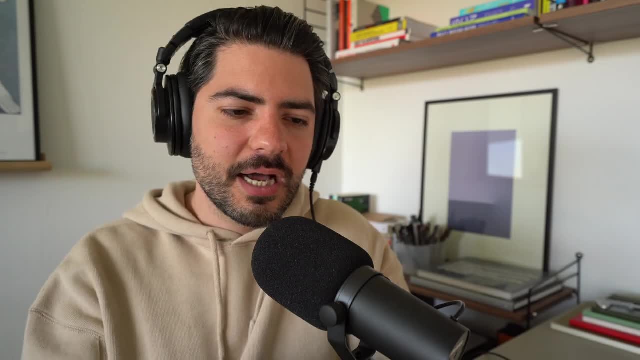 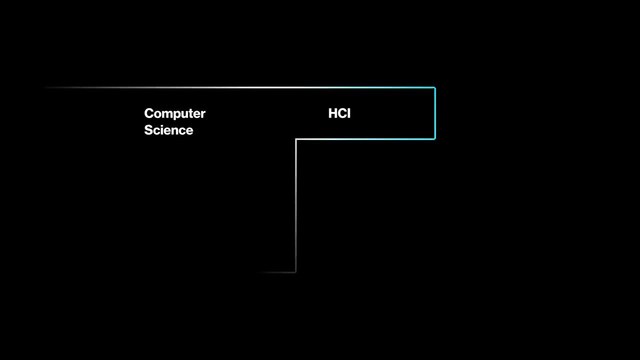 But after like 10 years of wading through all of those debates, I believe that I have come to an answer which is actually quite simple. The answer is that HCI is part of computer science. HCI is a part of computer science which builds on social sciences and humanities. 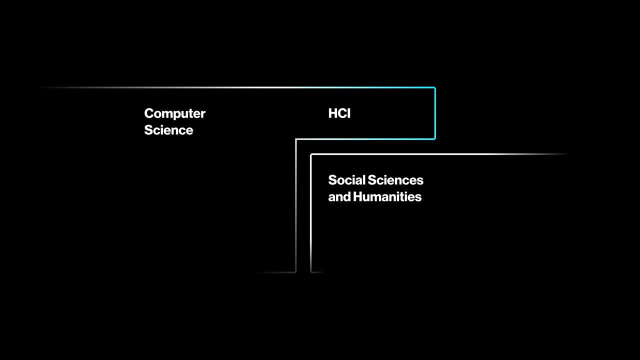 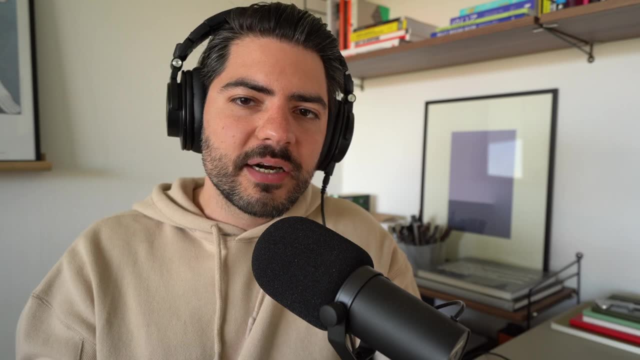 So let's talk about the two parts of this. First of all, the idea that HCI is a part of computer science, it's a subset of computer science, has to do with the fact of where it exists In practice. the absolute existential core of any scientific discipline today is publications. 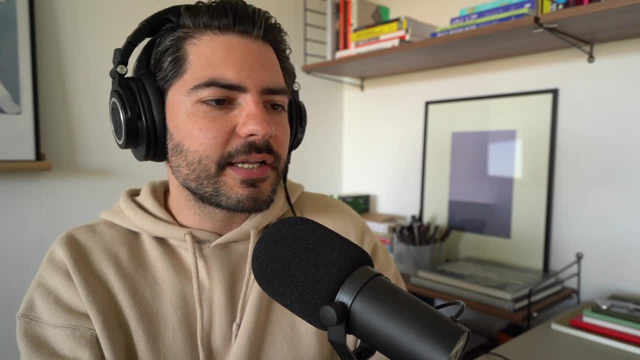 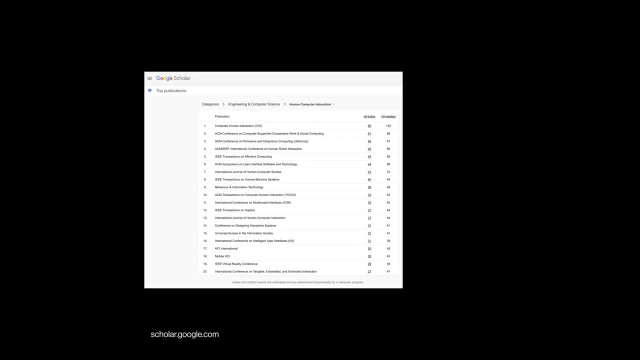 Any scientific field first of all exists as a collection of written documents. It's books or journal articles and conference papers. And if you look at the conferences and journals which define HCI, which are truly the infrastructure for the scientific community, these are produced. 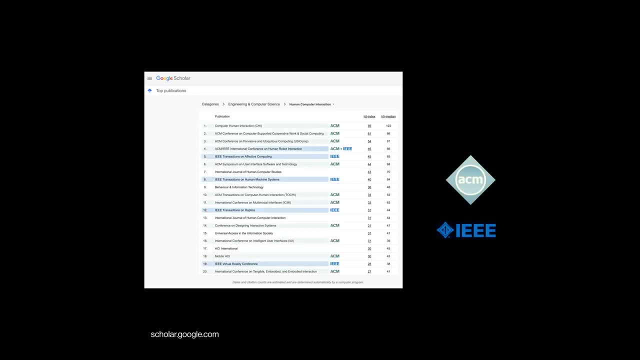 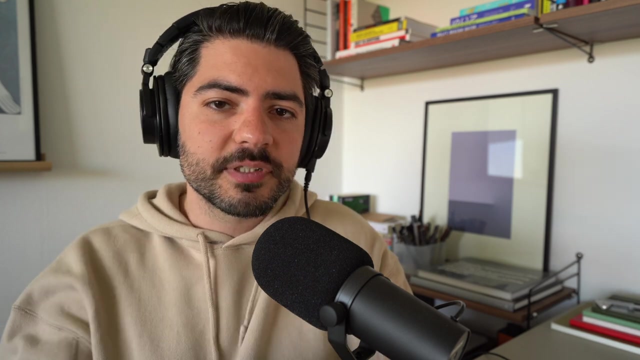 by organizations which define themselves in terms of computer science and engineering. The two largest ones are the ACM, or the Association for Computing Machinery, and IEEE, which is the Institute of Electrical and Electronics Engineers. Now people do argue that HCI extends beyond computer science, which it does. 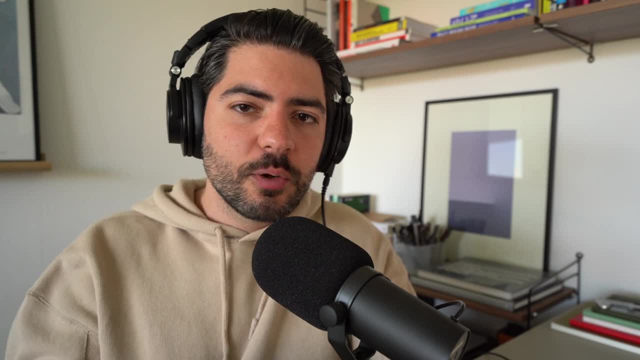 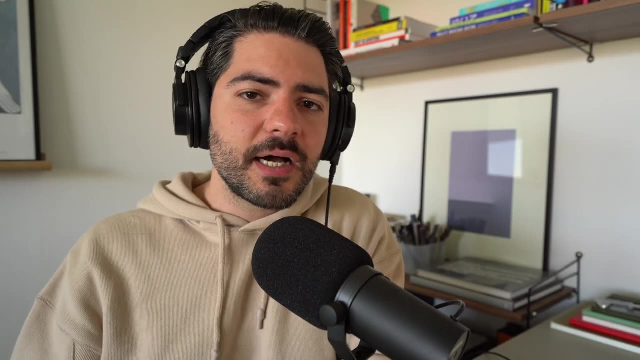 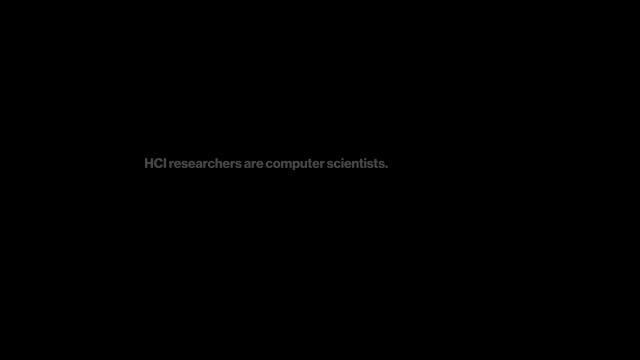 but my view is that when it does, it also extends the borders of computer science. It redefines what computer science is. But all of this philosophy aside, what follows for practical purposes is that being a HCI researcher means that you are a computer scientist. 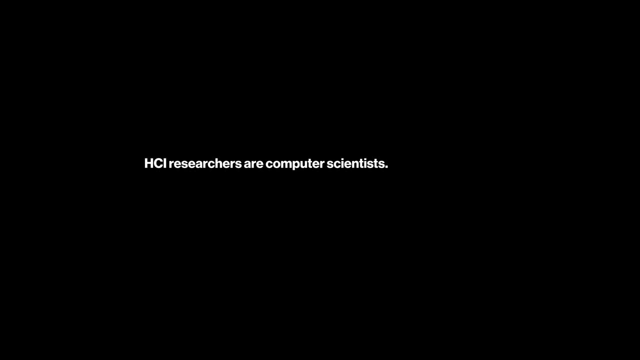 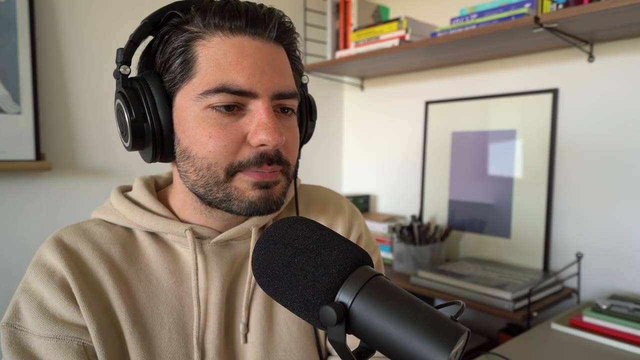 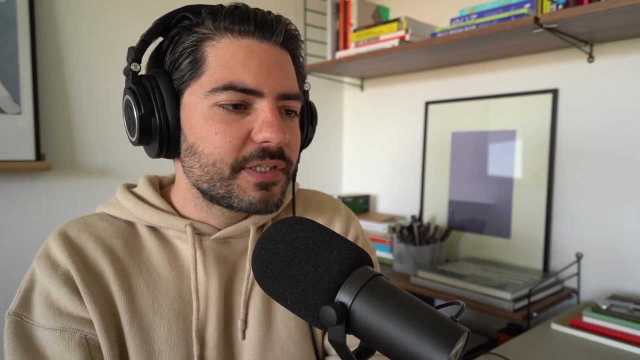 And if you are a computer scientist, then you will be expected to command the knowledge and skills that a competent computer scientist would possess. Even though in HCI you might specialize in methods and philosophies that come from elsewhere, your work is most probably going to involve computer science topics. 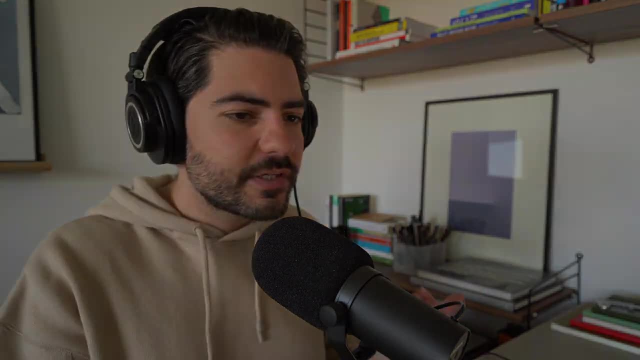 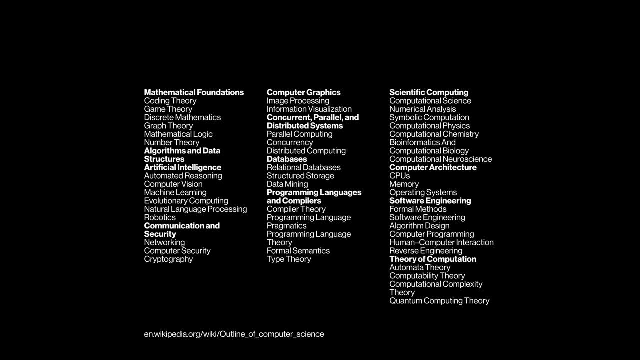 and you will have to have the competence to deal with these, like algorithms and data structures, information theory, graphics, signal processing, machine learning, electronics, software engineering. you can't avoid or outsource dealing with these topics as a HCI researcher. 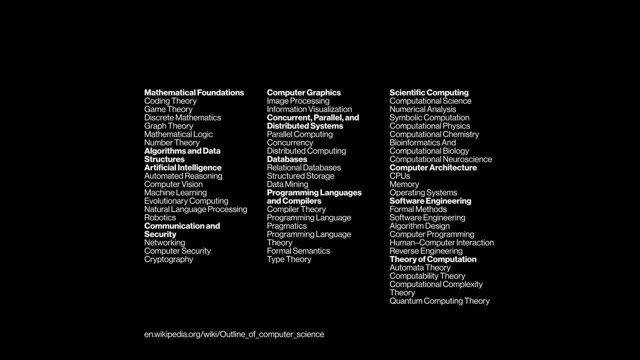 You don't have to be an expert on all of these, but in order to do your work you need to have a command of the basics, And, furthermore, many professors and other leaders who recruit for HCI research will have to be trained by a computer scientist, And so, in the 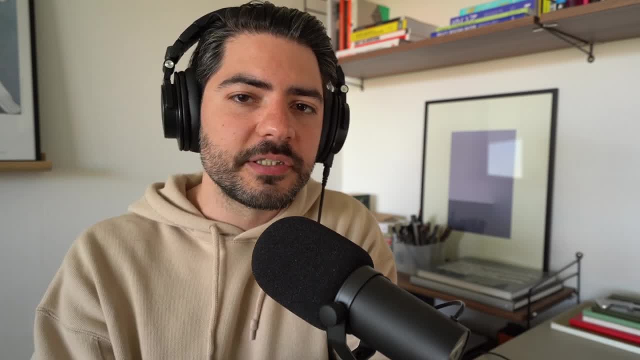 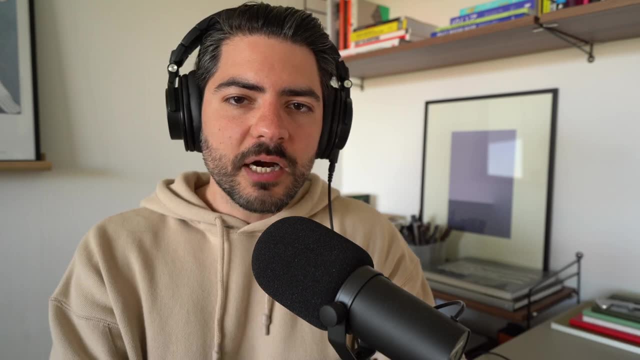 HCI related positions are themselves computer scientists and engineers, So being able to speak the same language as these people will carry you forward in the hiring process. So that's my argument, that for a career in HCI you really do need a strong foundation in computer science. 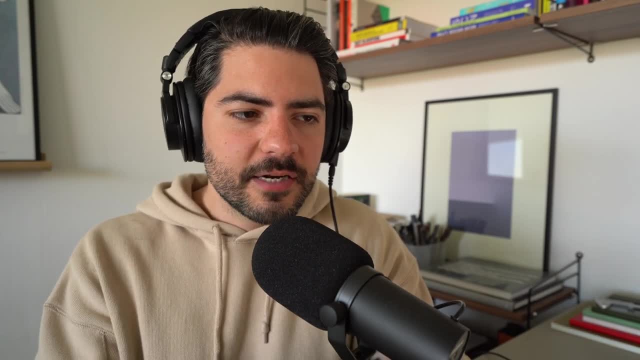 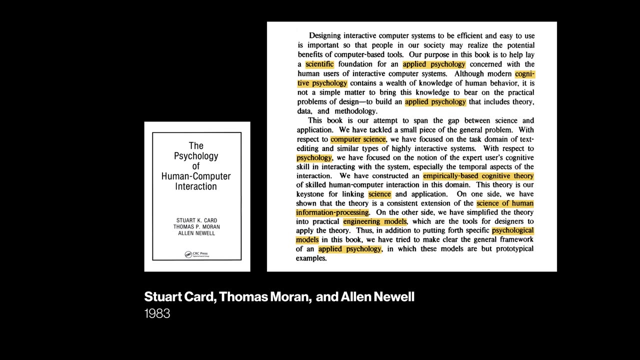 But there's one more thing you need, which is again a foundation and ideally a specialization in the social sciences and the humanities. I'm not going to go too deep into the history of HCI, which we might do in a future episode, But very briefly, the origin of HCI as a branch of computer. 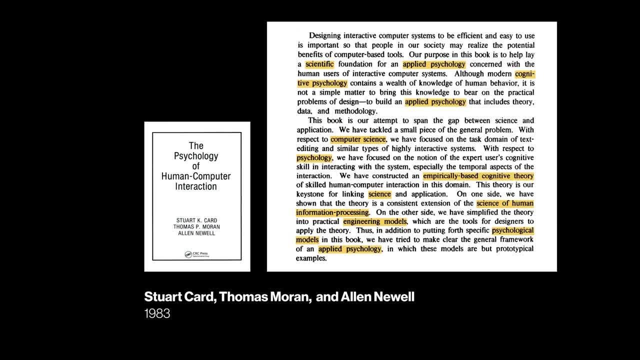 science really materializes in the 80s. There's a book from 1983, which really stands out. It's called The Psychology of Human-Computer Interaction And basically what's happening here is that the authors of this book are taking assumptions, methods, results and arguments from psychology. 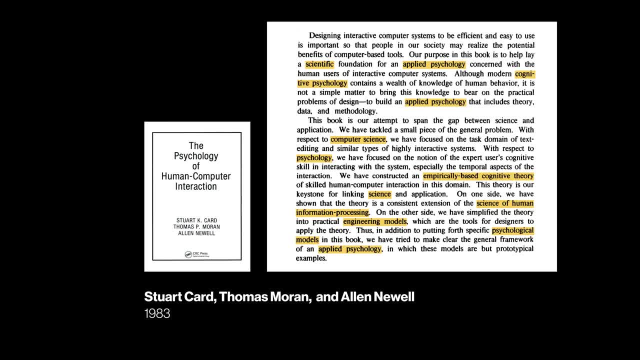 And from that they are deriving answers about how to design computers. So they expand computer science and psychology Towards each other. they kick off this interdisciplinary field called HCI, And over the years what happens is that people start bringing in other branches of social sciences. 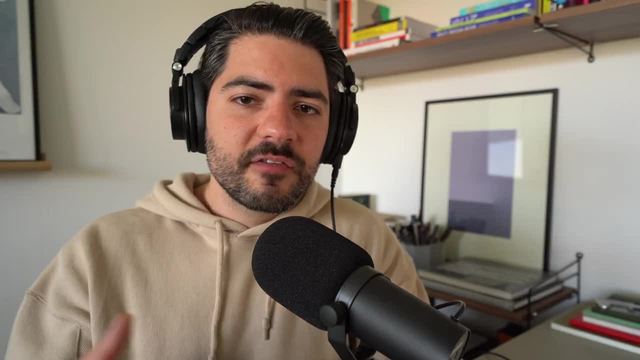 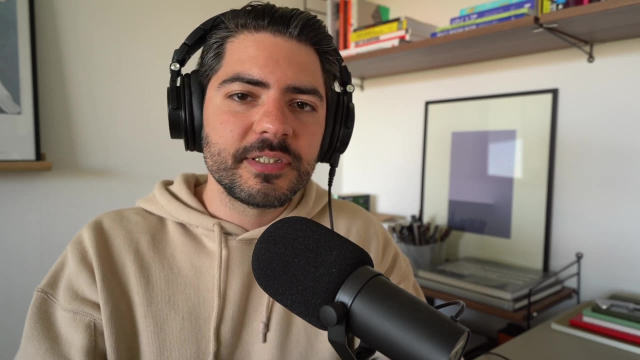 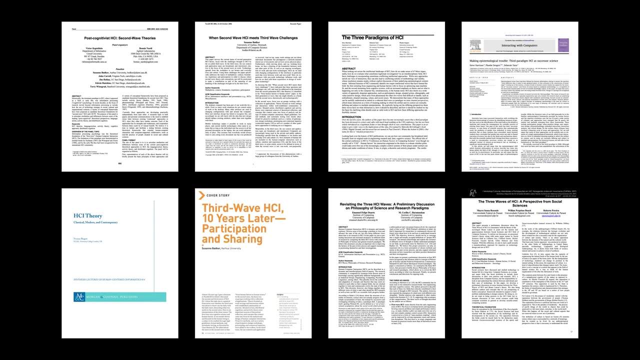 and humanities into HCI. If you actually get involved in HCI you will see that people talk about these three waves, or intellectual movements, that define its history and evolution. Psychology and computer science coming together is the first wave of HCI. The second wave is the rest of the 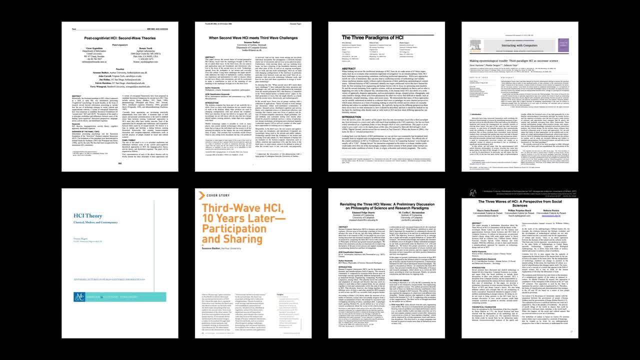 social sciences coming in Moving together with developments in computer technologies and devices and, of course, the internet. in order to deal with the new kinds of questions and possibilities that come from this technology, we bring assumptions and methods from disciplines like anthropology and sociology and media studies and more, and we're applying those to the phenomenon. 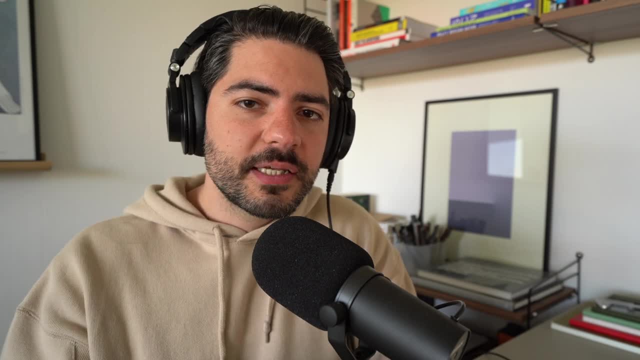 of HCI. So gradually a lot of new ways of thinking and doing research become accepted in HCI. The third wave of HCI is the process of thinking. The third wave of HCI is the process of understanding and change how we see the future Being in the space. we reveal ups and downs. AI adapts. 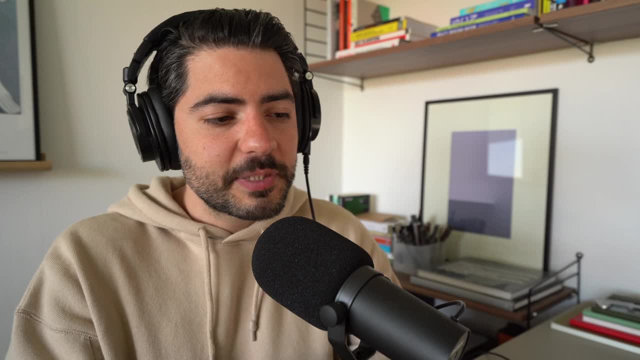 andHHH a number more. The third loop of HCI, though, is the process of becoming an independent and an independent person. HCI, then, is the same thing happening with humanities. As technology and computers become ingrained in our lives and the incredible ways we have today, it actually becomes possible. 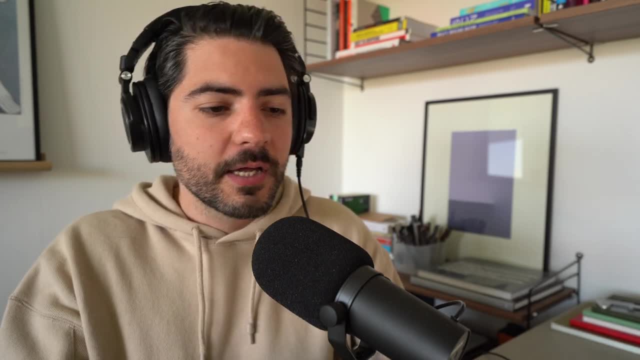 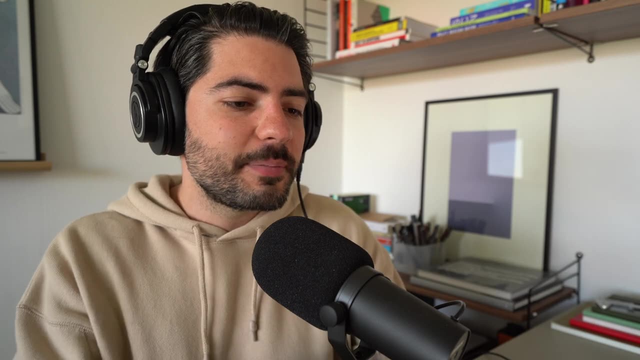 and even necessary to use methods and philosophy like literature, philosophy, critical theory, arts and, of course, design, in order to make sense of the plays and the possibilities of computers in our lives. What HCI was initially intended to be- enjoyment and purpose, which would allready go under. 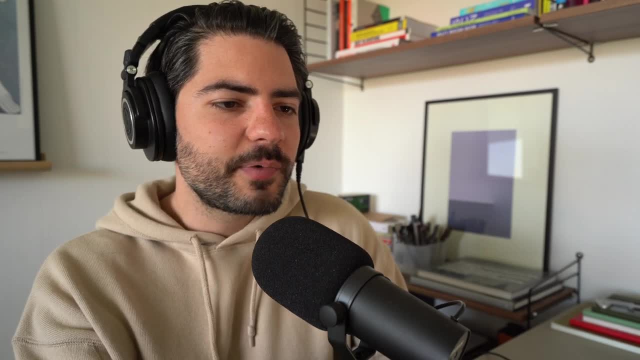 HCI was concretelyอะ him prop demographics of the last century, and far more so that it would be also considered as ascenesfor a future that otherwise couldstage low polish, and�� it became a new form of inclusion. it was was mating managers which would then run. 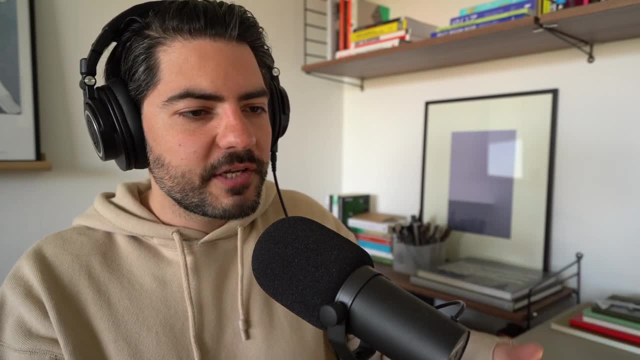 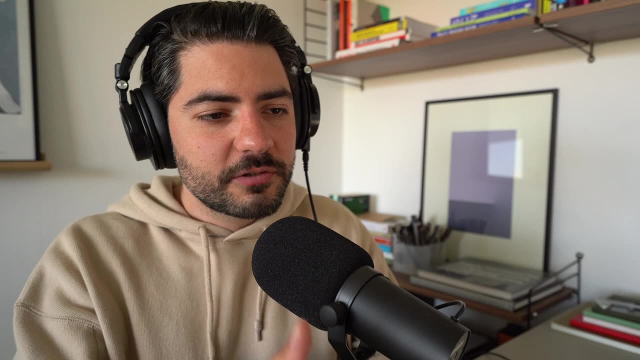 science, where we take knowledge and methods or, if you want to be technical about it, we take the epistemologies and methodologies from schools of thought which traditionally have nothing to do with computer science, And we use them to figure out how to deal with all of this technology. 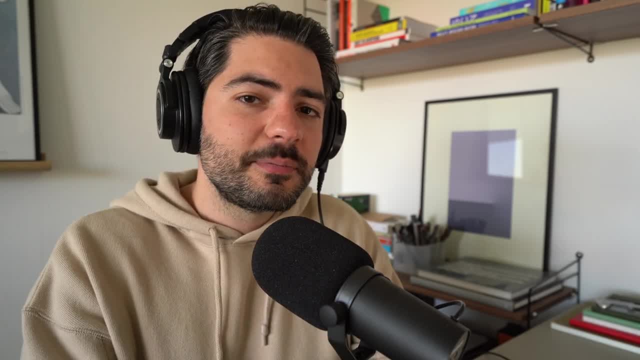 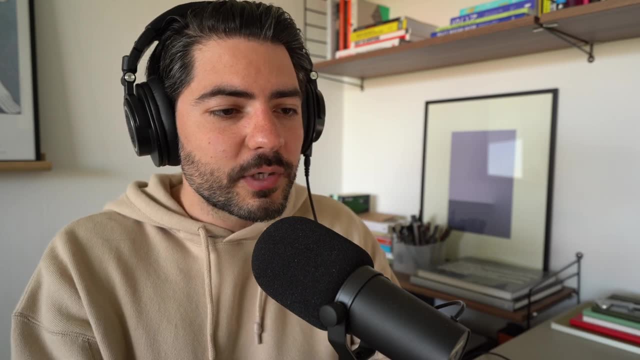 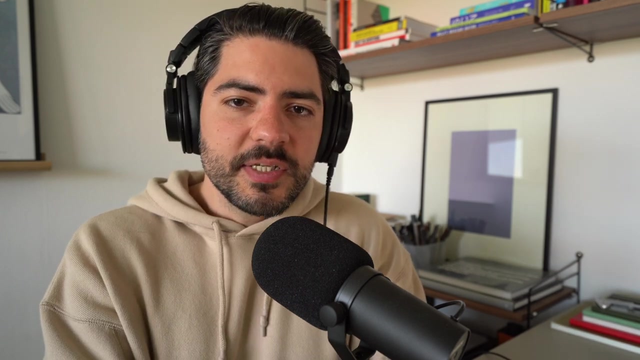 It's a very fortunate, very beautiful place to be And, having learned from this history, HCI today is a very tolerant, very inclusive place where ideas that might not initially make sense to computer scientists might get accepted. And this brings me to my final point, because this: 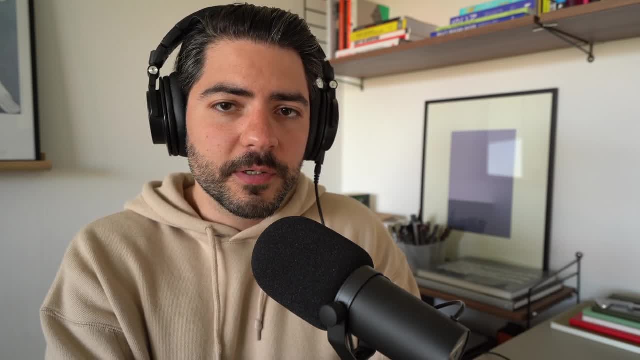 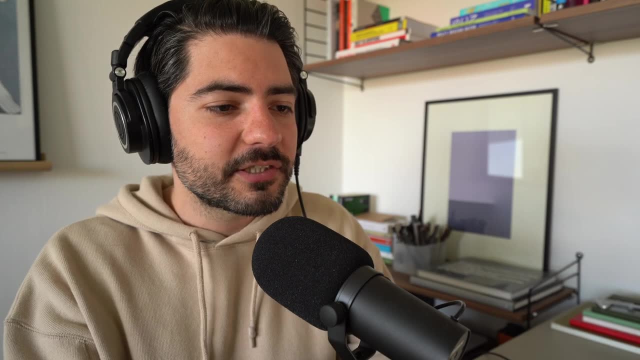 tolerance and inclusivity is a double-edged sword. On one hand, it allows us to consider unconventional ideas, it frees us from prejudice, and it paves the way to innovation and invention, Not to mention that it creates a beautiful community where all kinds of individuals 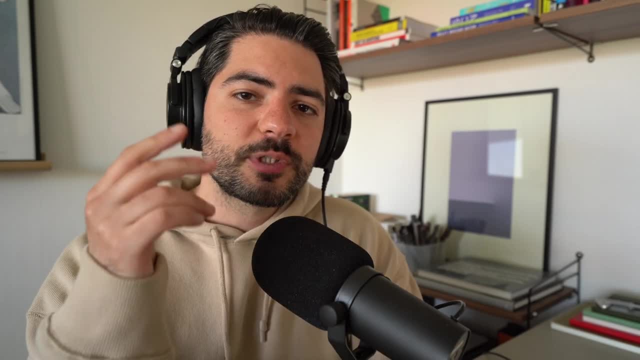 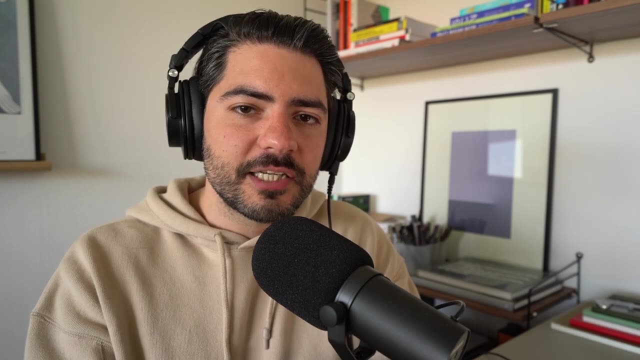 are accepted. On the other hand, it certainly makes it difficult for outsiders and beginners to make sense of what we're doing, And it makes it difficult for us to have standards and recognize really high quality and really meaningful work. So what does this mean for someone who's interested? 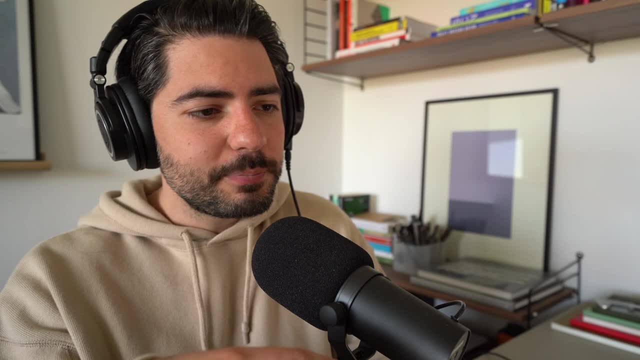 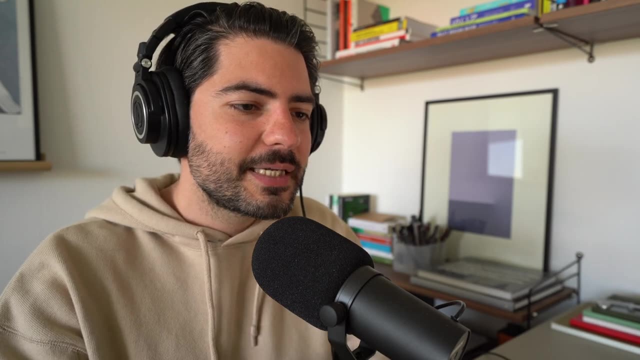 in joining the world of HCI. Well, it means that, in addition to being a citizen of the academic world and mastering its rituals, in addition to being a competent computer scientist, there is a third area of competence which you need to master, And that is the ability to 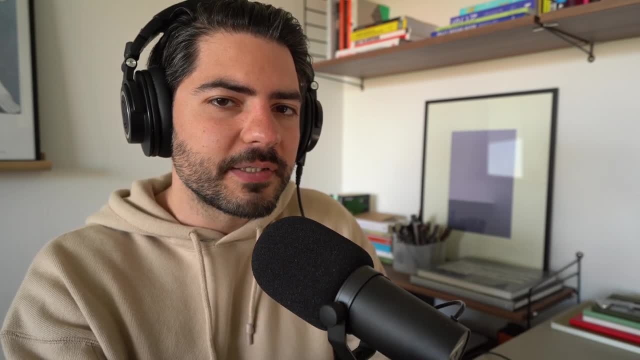 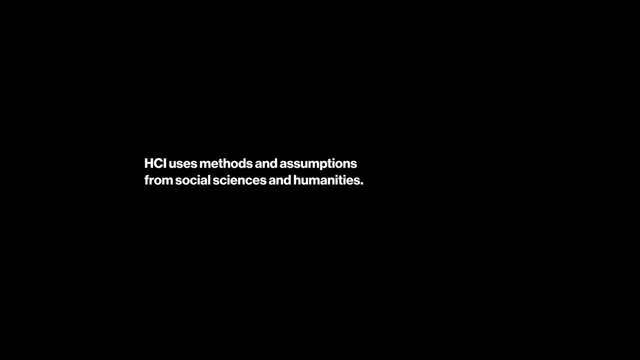 command, and this is the social sciences and humanities. Now, you don't need to be a master of the entire landscape here, although it definitely pays off to have like knowledge of the whole spectrum. But when you come into HCI you should come equipped with, let's say, 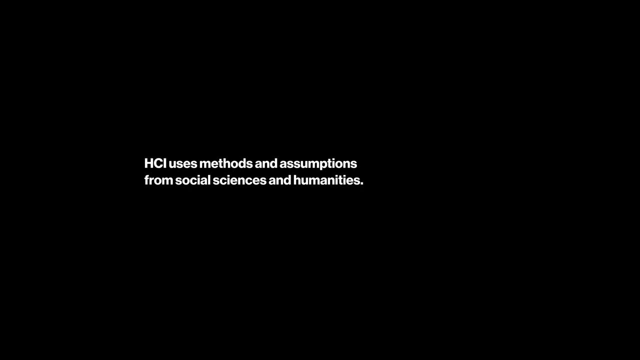 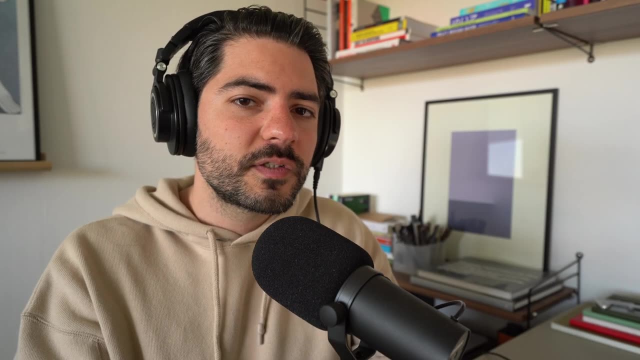 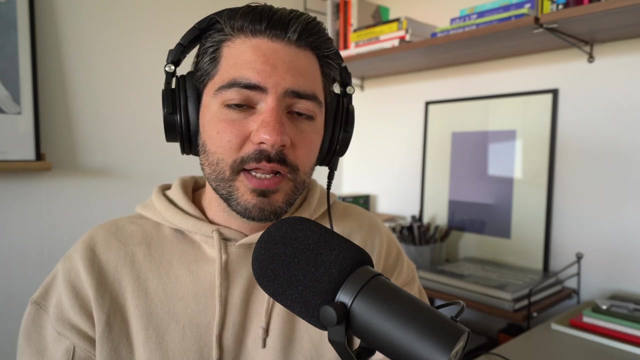 the equivalent of a university degree in terms of your skill and competence in one of those fields like psychology or anthropology or critical theory or sociology and, of course, design. I know that this is a lot of work. it takes many years to cultivate this competence in computer science as well as, let's say, anthropology, And this exactly is the reason. 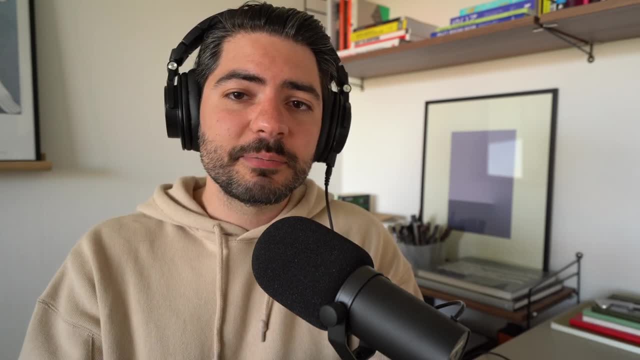 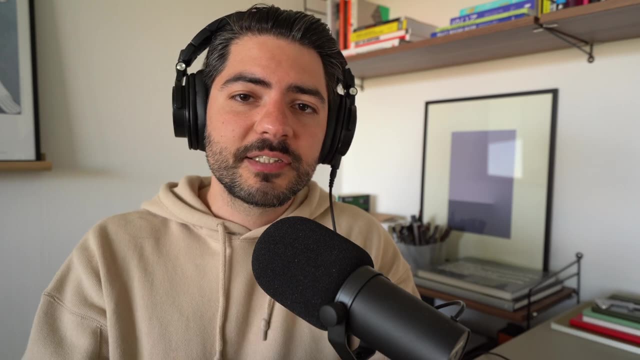 why most HCI schools are graduate level. they are masters and PhD programs, because this gives you the time to cultivate these skills and also familiarize with the rest of the academic ecosystem in the previous years of your schooling. But going back to the question of what you will, 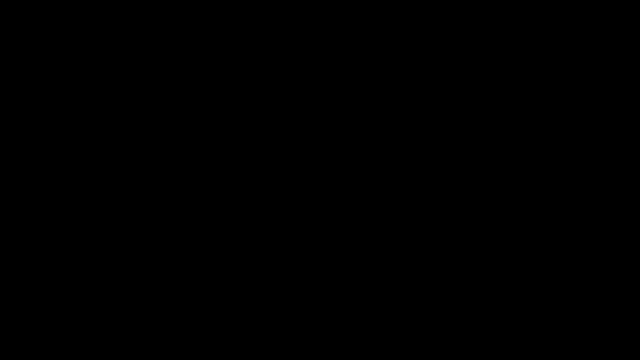 need in HCI if you have this combination of skills, which is first of all an interest in academic research and then competence in computer science, and then also the ability to develop your skills in computer science and then a branch of social sciences or humanities. 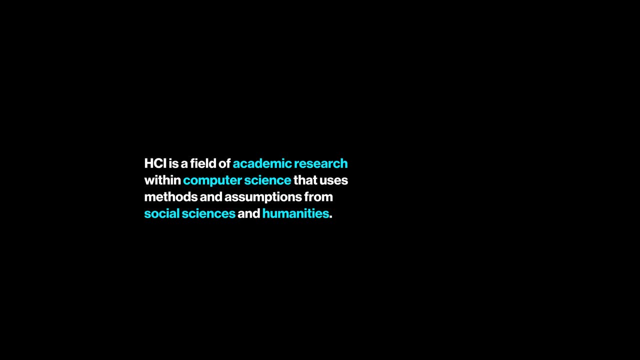 including, but not limited to, some kind of design discipline, And maybe you can add to that the specific things that your project or your team might specialize in. you will be unstoppable. you'll have no problem getting into a HCI program. you'll have no problem going through it. 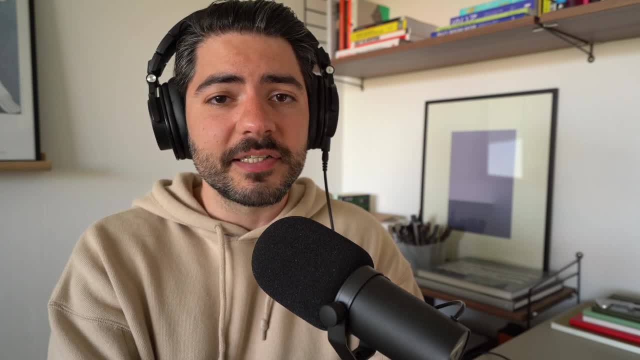 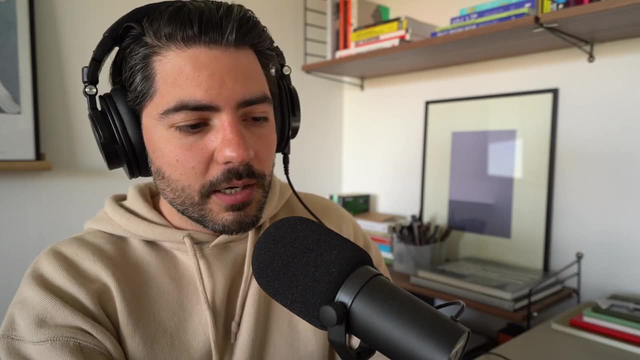 and you'll have no problem succeeding in the rest of your career as a HCI professional If you've been looking at HCI programs- or maybe you're already in a HCI school and you realize there are parts of this combination of topics that you're not really super excited about. 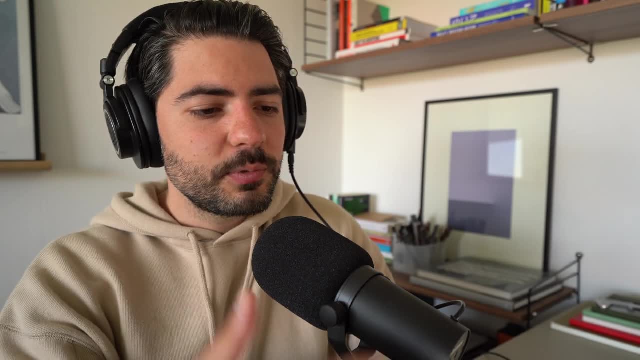 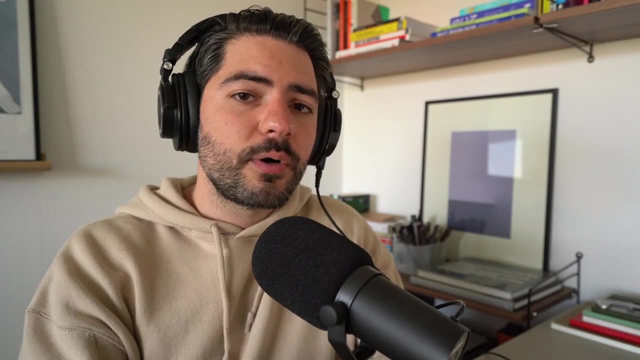 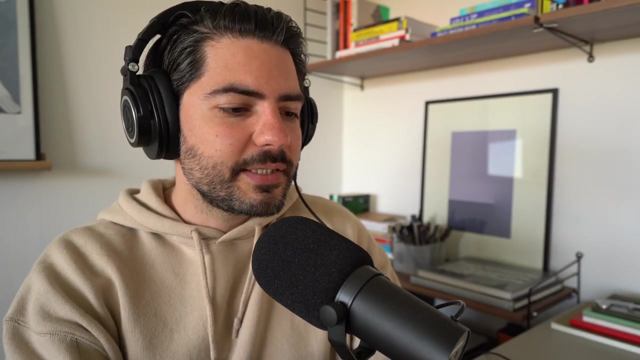 that's actually totally fine. You can find projects and team up with people where you focus on maybe software development, maybe graphic design, maybe ethnographic research, whatever you enjoy. But simply realizing that HCI is the name of a branch of computer science, research which brings in the social sciences and humanities, allows you to make sense of things. 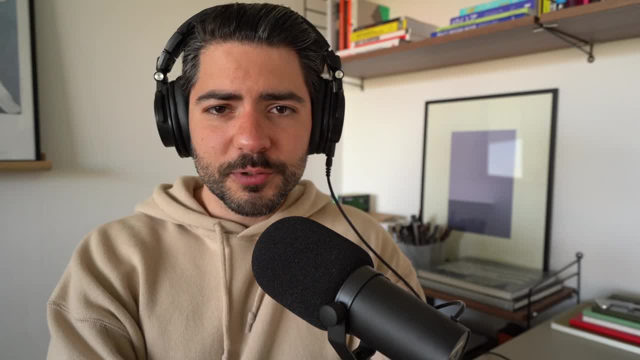 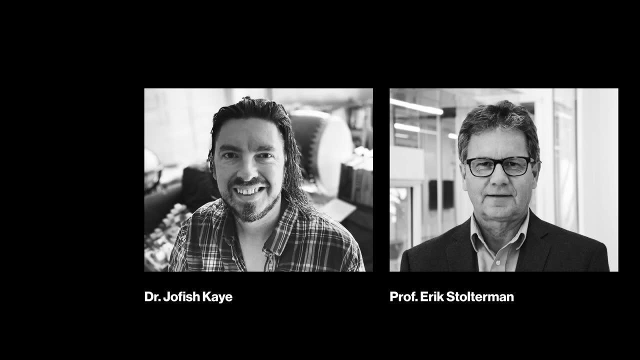 and make faster and easier progress. In future episodes of Design Discipline, we're going to continue to explore the world of HCI. We have already had guests like Joe Fischke and Erik Stoltermann, who have had very successful and very different careers in this world. We are going to have many.